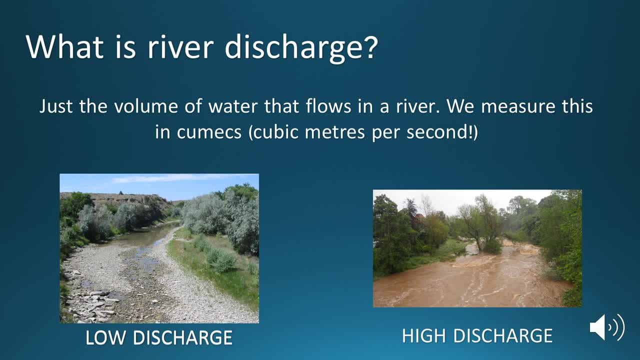 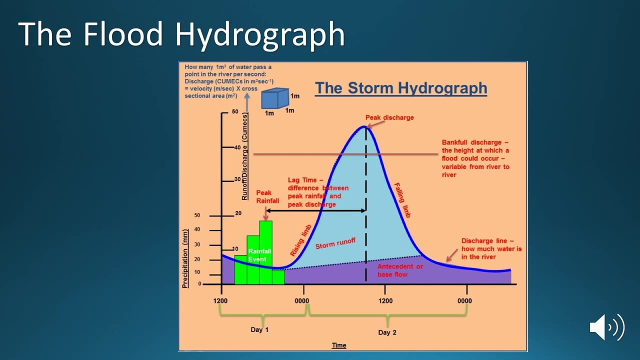 So, therefore, you would expect there to be a high number of cubic meters flowing past a given point every second. So, in order to assess flood risk actually, and to assess essentially how quickly rainfall enters a river channel, we use something called a storm hydrograph. So I'm going to talk you through the 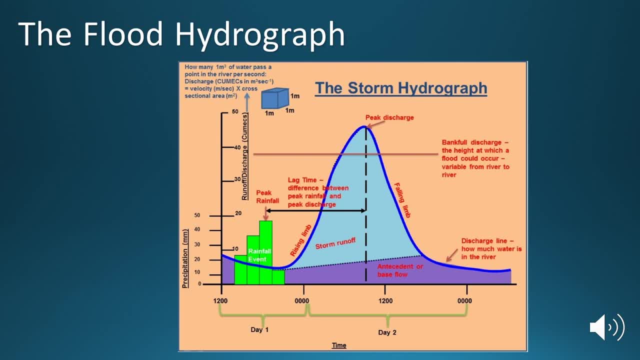 very basics. I'm going to talk you through from start to finish of how you would interpret one of these graphs. So let's look at the axes to start off with, and we'll start off with the y-axis, that vertical axis. Now, the y-axis is the vertical axis of the river. So if you look at the y-axis, 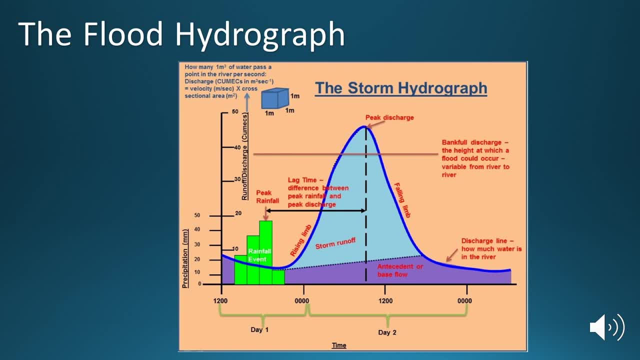 there are two things that we can read from this. First, precipitation, which we're measuring in millimetres, and you can see that at the bottom of the axes, precipitation from 0 to 50 millimetres. That corresponds to the bar chart, that light green and that very bright light green bar chart. 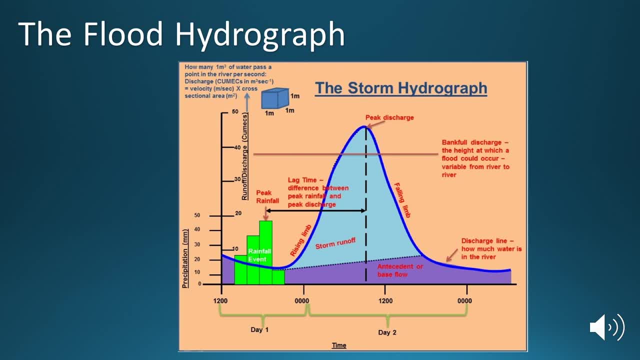 and that shows us how much rainfall we've had and when we've actually had the rainfall itself. So you can measure that. so, for example, that first bar looks to me something like around about 21,, 21,, 22- sorry, 21 to 22 millimetres of precipitation. 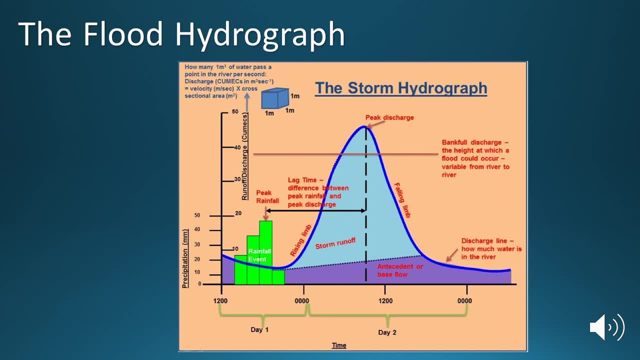 And we can see that the peak rainfall, by the maximum amount of rainfall that fell, was on that third bar and that was around about 45 millimetres of rainfall. So we can see how much rainfalls fell and when it's fell, which is very important for our flood risk. Second thing: we can 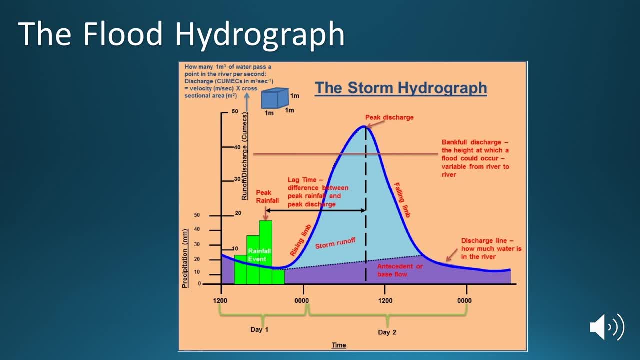 measure on the y-axis is the runoff slash river discharge, which we measure in cumecs, And you can see that going from 0 to 10,, 20,, 30,, 40, 50 using the full extent of the y-axis And 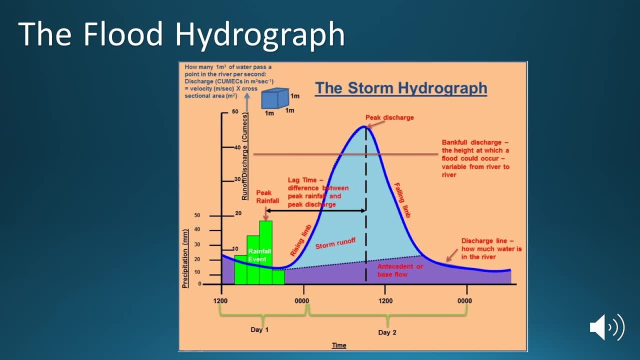 that corresponds to the line graph that you can see, and the line graph you can see is in dark blue. So if we run through this, we can see that to start off with at 12 o'clock- along the bottom we're working in time, sorry. along the x-axis we can see that we get a slight decrease and then we get an. 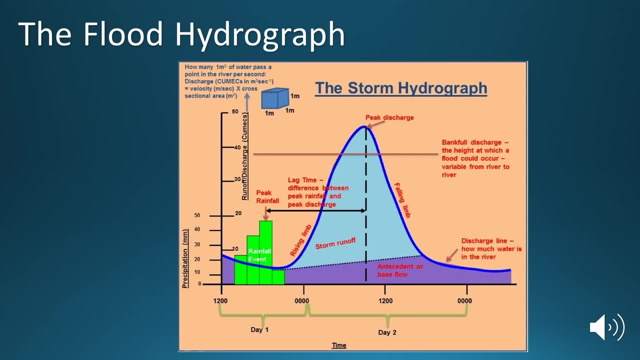 increase in river discharge up to the peak, a decrease in river discharge and then a flattening out of the curve back to normal levels. So let's talk through and run through each of these stages. So if we move to the line graph, we can see that that corresponds with an increase. 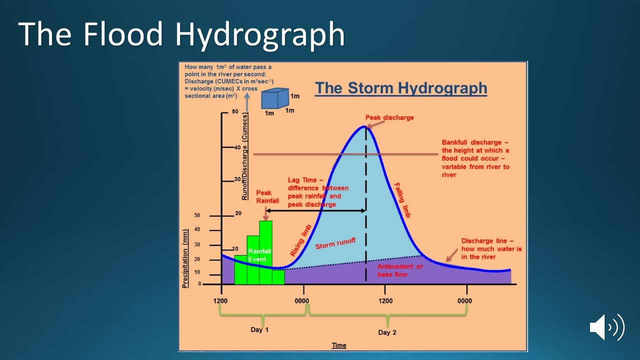 a couple of hours later, in river discharge within the river system, the river channel itself. Now this increase we call the rising limb. So the rising limb is the word we use to describe the increase in river discharge. you see on the storm hydrograph And this continues to increase. 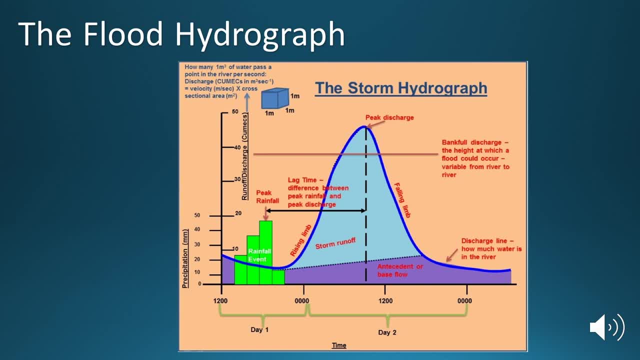 up until we get to something called peak discharge, ie the maximum amount of water in the river channel at a given time. The peak discharge, the maximum amount of discharge that we get. So we get peak discharge and then we start to get a decrease and as that decreases we call 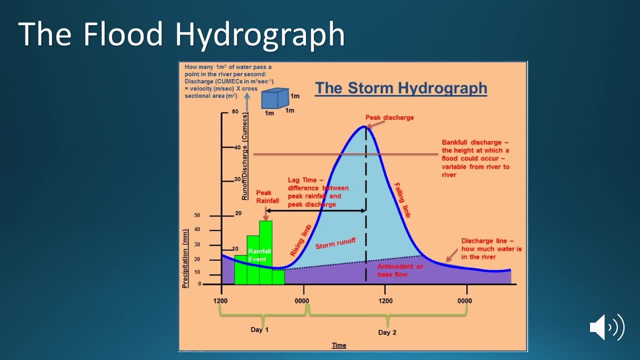 that the falling limb, the opposite to the rising limb. it's falling, the discharge is falling, okay, So we get a falling limb decrease in river discharge and we get back to the point where we are kind of normal conditions. So, as you say, that dark blue line is the 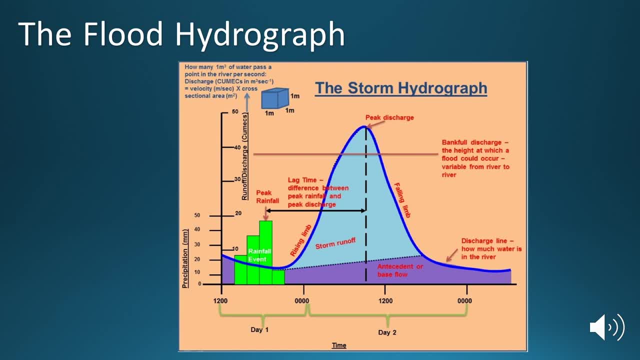 discharge line. this is just showing us how much water is actually in the river at any given time. An increase is called the rising limb. It's a peak discharge and it will decrease. and then it's a falling limb, So we get a decrease in river discharge. 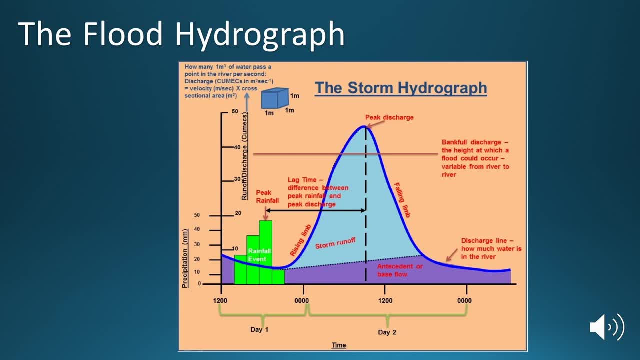 and it will decrease and then it's a falling limb. So we get a decrease and it's a falling limb. Now let's look at the peak discharge and the peak rainfall. We can calculate the time difference between those. So, looking at this graph, the peak rainfall looked to have occurred at maybe around. 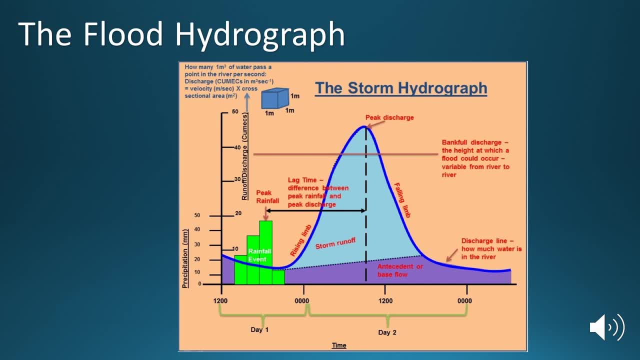 about seven or eight o'clock, something like that, And peak discharge looks to have occurred at around about 10 o'clock, something like that. So we can calculate the difference in time or the amount peak rainfall to occur and the peak discharge to occur, and that essentially tells us how long it. 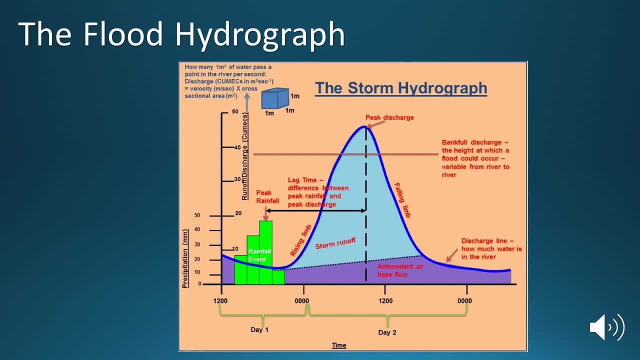 takes for the rainfall to fall- ie rainfall or precipitation- and for it to then move through the grain system and flow and arrive into the river channel. so that's the lag time. that's probably the most important measurement that we get from the storm hydrograph. so how long does it? 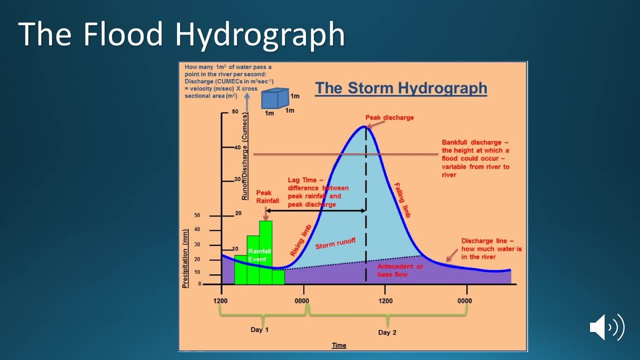 take for the rainfall to enter the river system. now, with the terms that we've got on here, that i haven't described yet, we've got the antecedent or base flow, which is along the bottom, that purple colour. now antecedent again is a post-scientific word for the conditions that occurred before. so